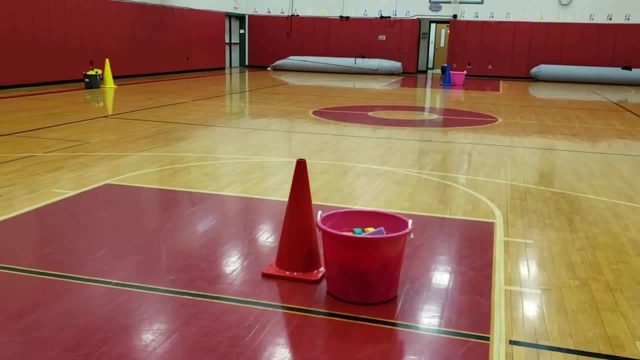 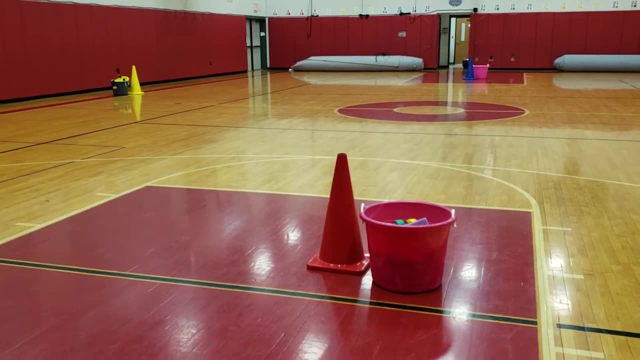 All right, going to take you through some kindergarten stations I'm doing today. I've done stations more than ever this year with this group and it has worked really well. I've got about 30 kids and very much varying abilities all throughout and these have worked really well. 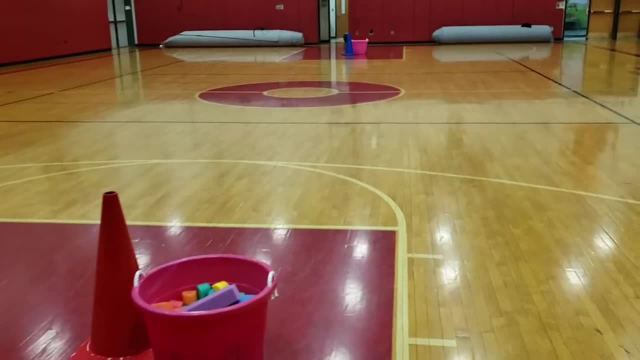 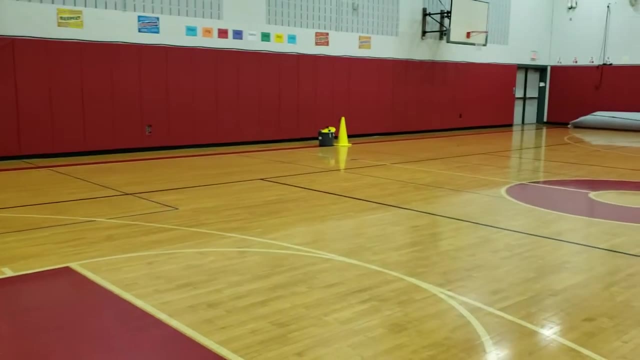 So six different stations with six different objectives. So the first one- and they're all really, really simple- You could probably pull off with about any kind of equipment. So the first one is just a little teamwork challenge Here. we just have a bunch of random stuff. 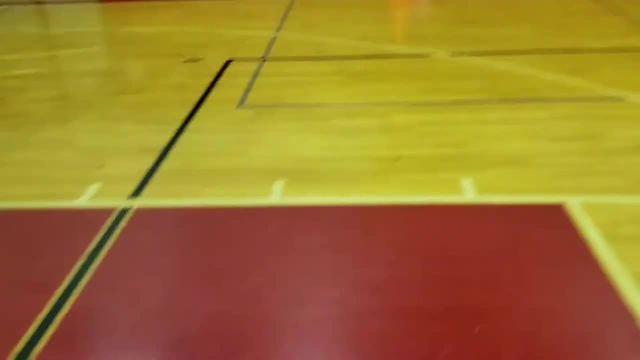 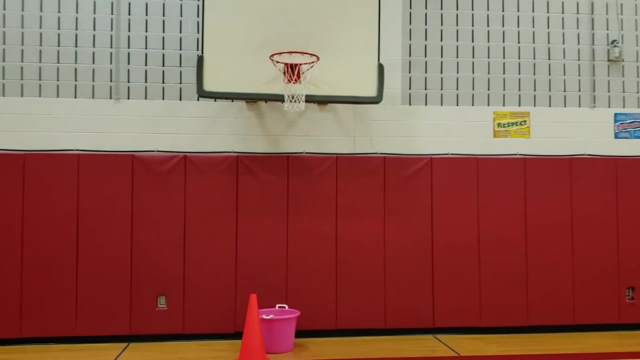 They're going to build the biggest tower that they can. Next one is going to be some type of throwing challenge. This one, we have some Frisbees and they're going to try to get it in the basket. This basket's set at, this one's at nine feet. 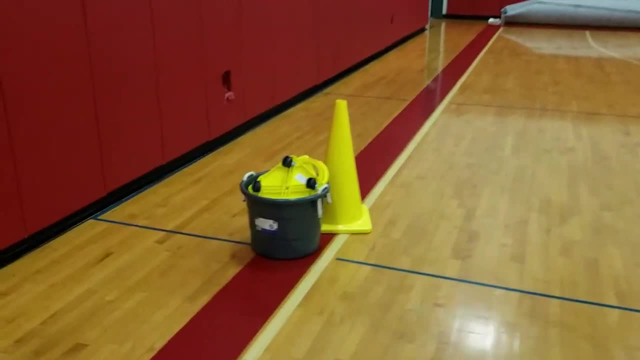 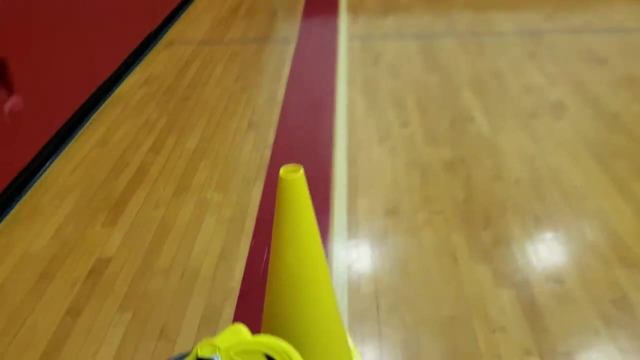 They've had no problem getting it up there. Next one is some type of balance station. Today it's scooters, but we've had the hilltops, The stepchairs, The stepping stones and the Spooner boards mixing in at this station and that's worked good. 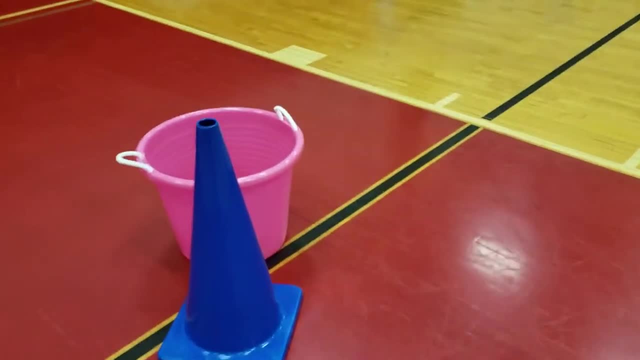 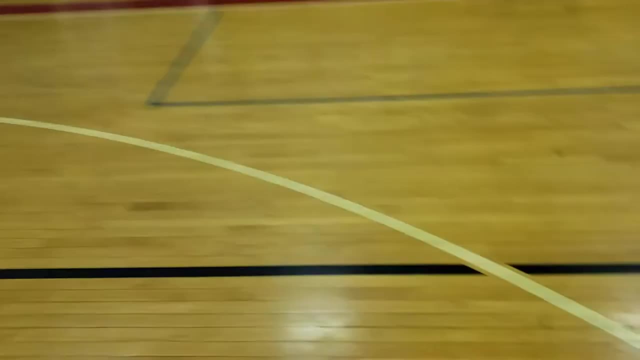 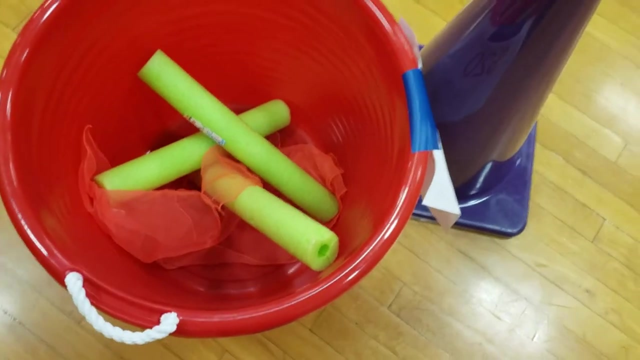 Over here we have some type of striking station. Today we have just some balloons that they're going to be hitting up to themselves. I've used noodles and paddles there. Also, over here it's a tracking challenge, So they're going to toss a scarf up in the air and then try to catch it on top of the noodle piece. noodle cut up noodle pieces. 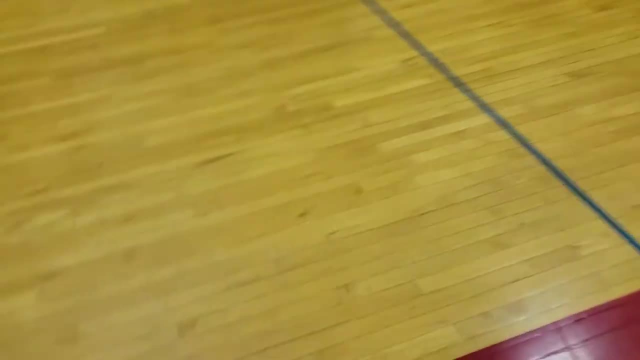 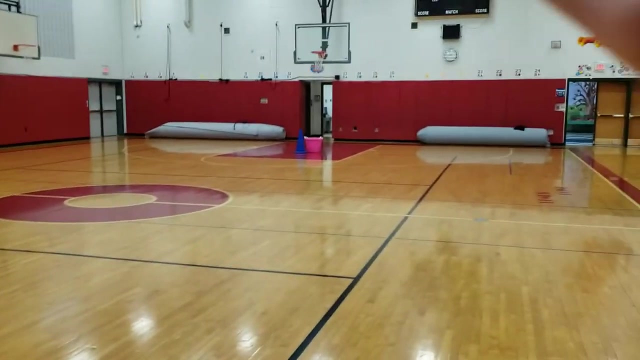 And then we have a kicking challenge. So simple: kick the soccer ball from the red line, try to get it into the goal. So six stations: teamwork, throwing, balance striking, tracking, kicking- So we kind of meet a little bit of everything. 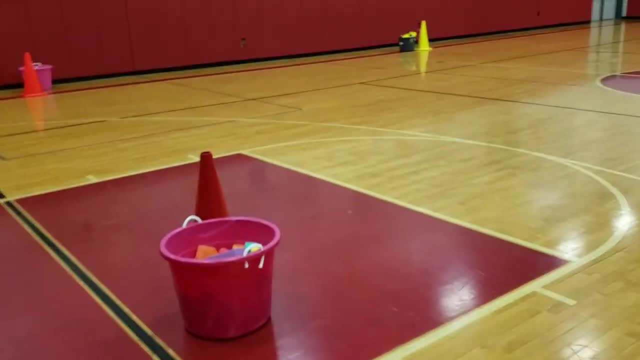 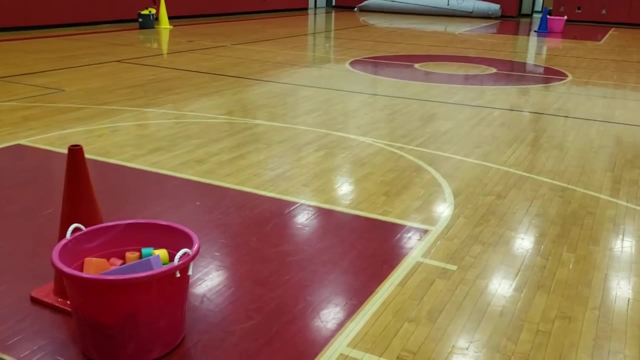 We definitely work on the transitions. What I do is when I say one, two, three, clean up. students put everything from their station inside their bucket and then sit back-to-back with their partners and point to the next station. We practice that a bunch so they have that down. But definitely need to make sure that's clear. All right, thanks.